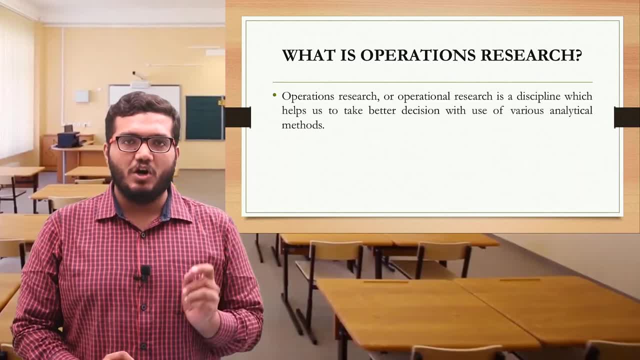 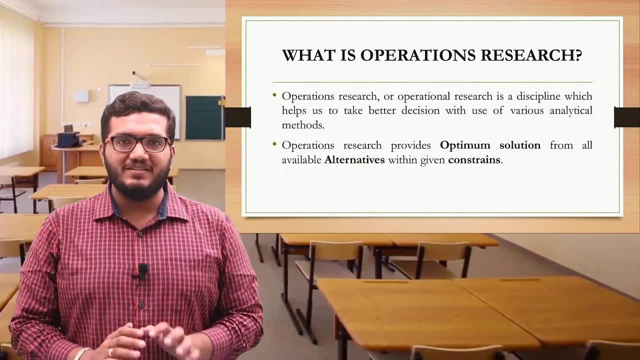 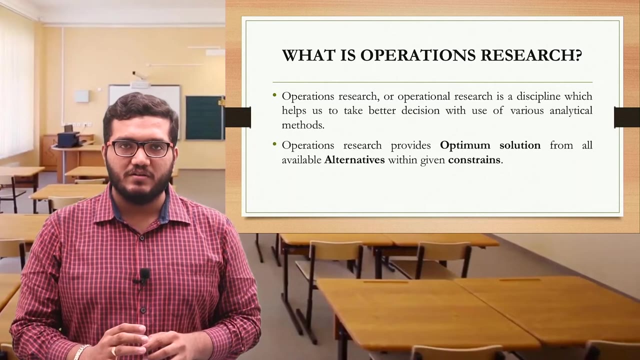 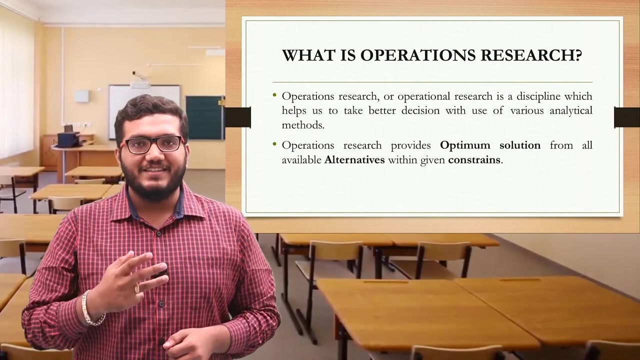 And it must be the optimum in terms of maximization or minimization, Operation Research, that provide us the first step. It is the facility to optimum our function by considering the various alternatives and the constraints that we have. Here we are having three different terms. 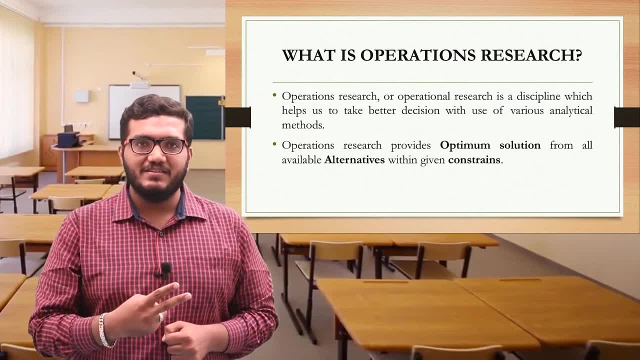 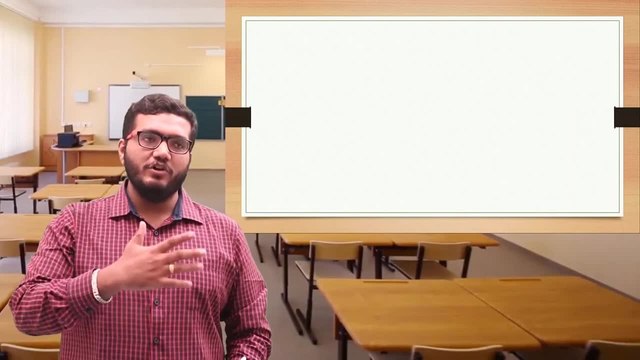 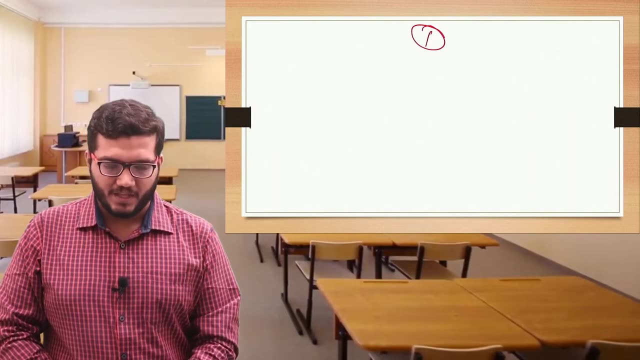 The first term is objective function, the second is constraint and the third is alternatives. So let us take one example: If I want to travel from city 1 to city 2.. So here we are having the first city And this is our second city. 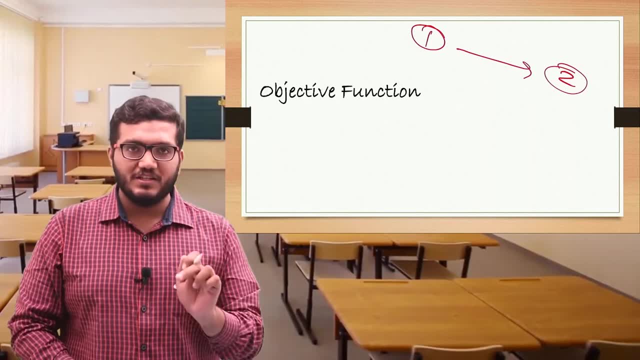 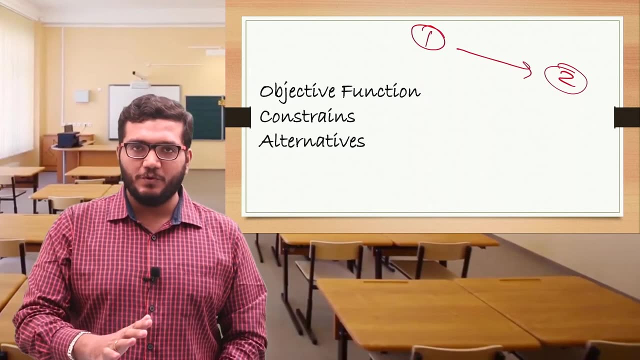 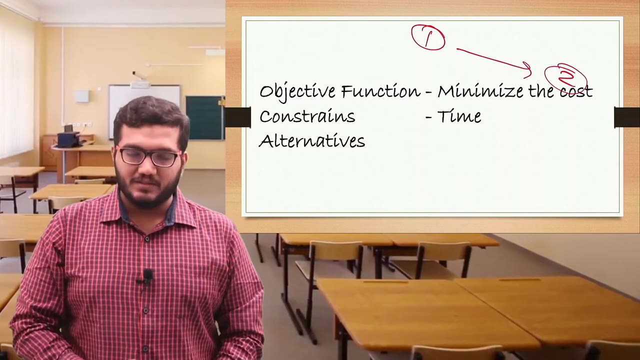 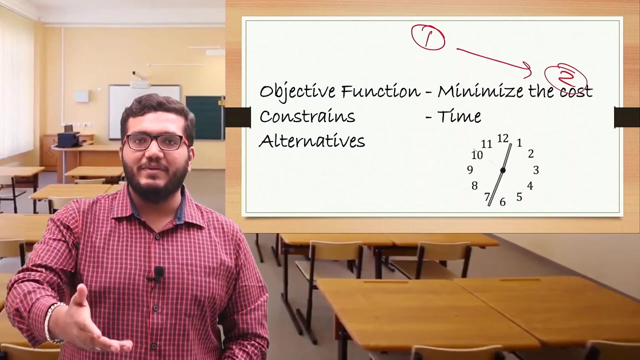 Now what I need to define is the first is objective function, second is constraint and the third thing is alternative For this problem. my objective function is to minimizing the cost, the cost of transportation. The constraint that I have is the time I need to reach before 10 am, as my meeting is scheduled on the next day morning 10 am. 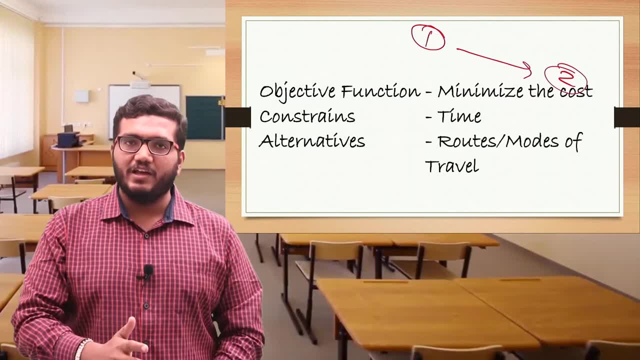 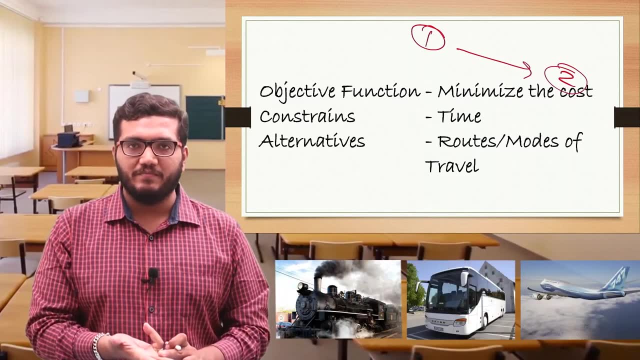 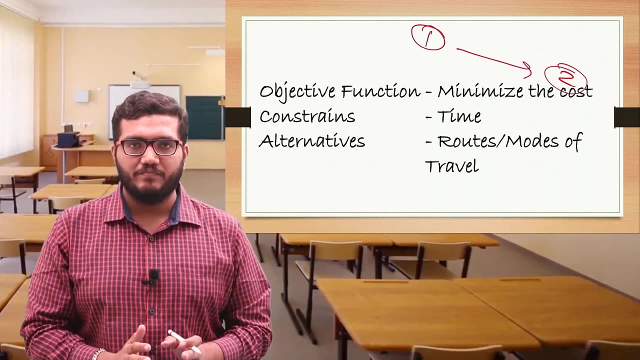 And the third. the third alternative that I have is the different routes I can go, the different mode of travel, like by train, by bus, by plane. So these are the three basic terminology that we are going to use in operation research. The next is the phases of operation research. 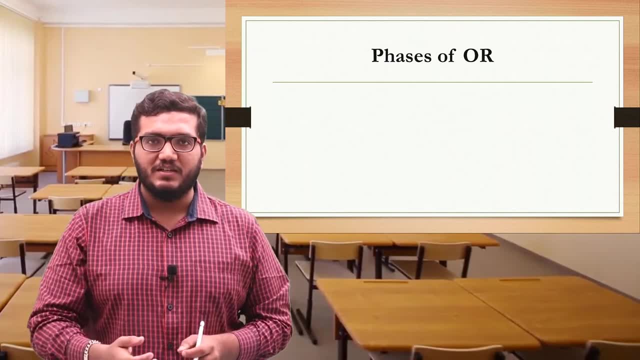 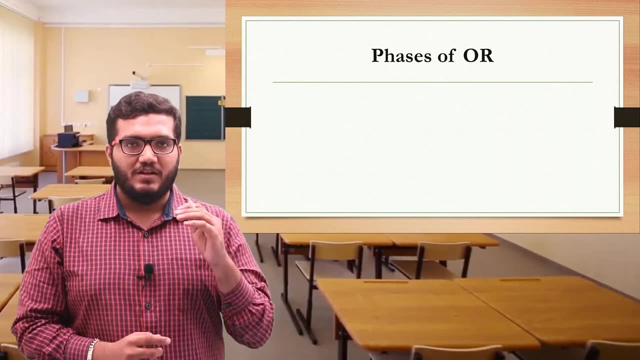 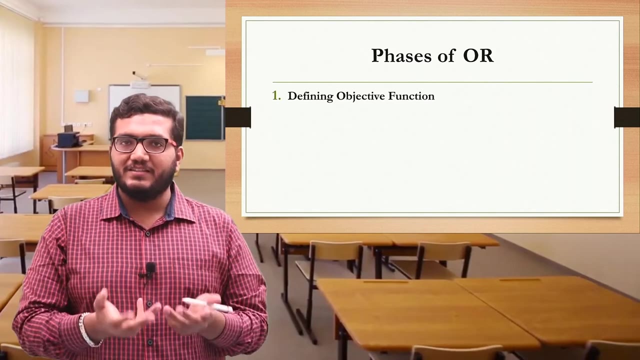 When we are talking about the phases of operation research. that means how the operation research is going to provide us the solution. The very first and the basic step of operation research is defining our objective function. There are three different types of objective function. The first is maximization type. 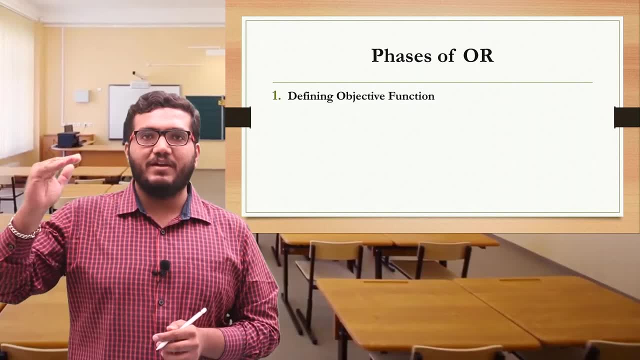 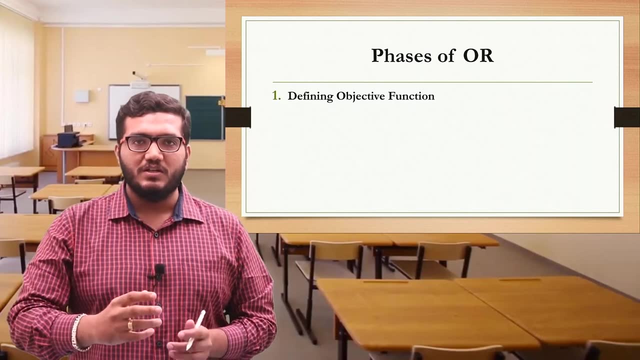 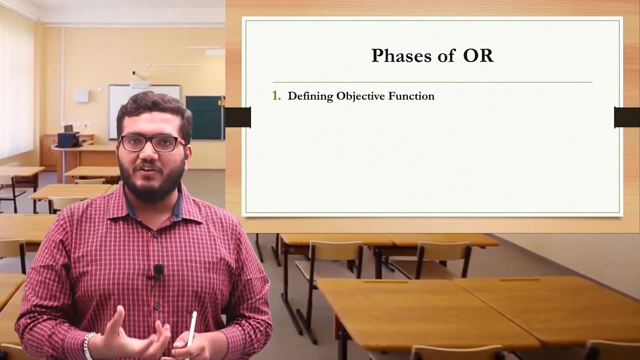 If I am talking about the profit, I need to maximize my profit. The second objective function is of minimization type If I am talking about the transportation cost, so I am always looking to minimize my transportation cost. And the third is If I am suffering from sugar, so my sugar levels need to be maintained within certain limit. 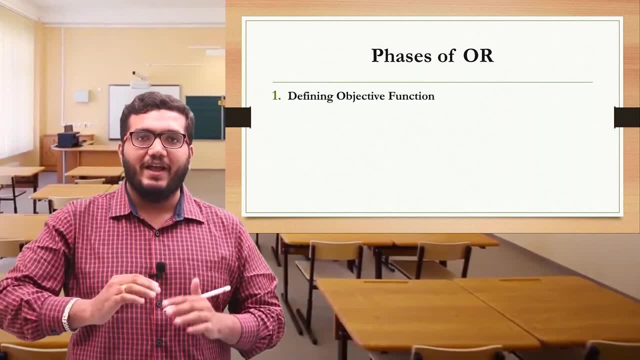 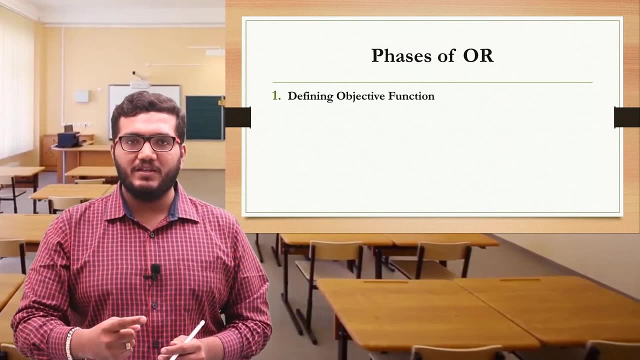 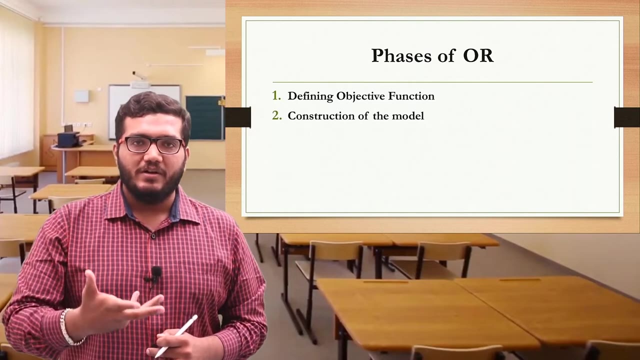 Not below the certain limit. not above the certain limit, And in this case I need to optimize my objective function. So the very first step is defining my objective function. After defining objective function, I am going to develop my model. So the second is construction of model. 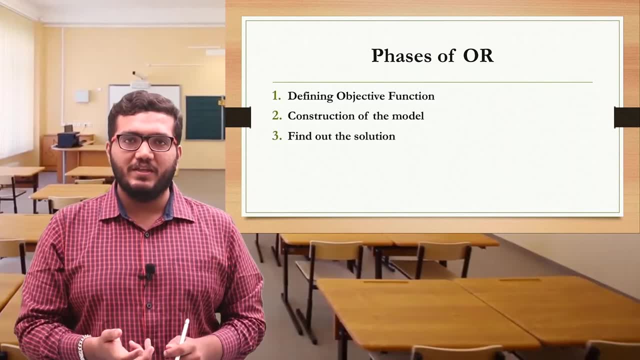 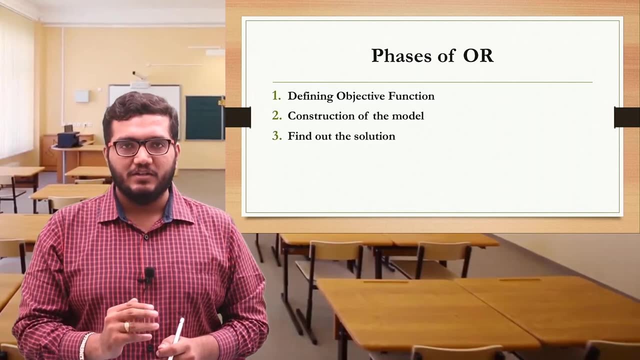 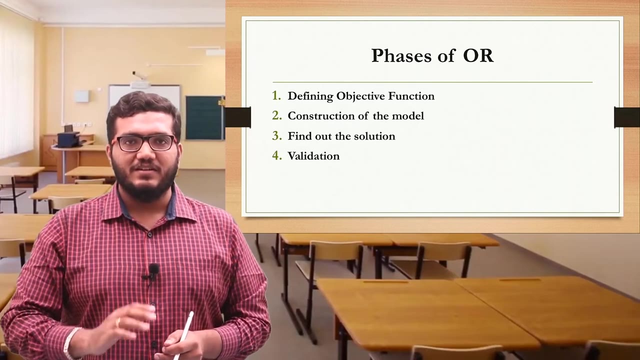 After constructing my model, the third step is finding out the solution. When I am going to find out the solution, I need to validate it. So the validation is my fourth step And, after the validation, the final stage, that is implementation, The implementation in the real life. 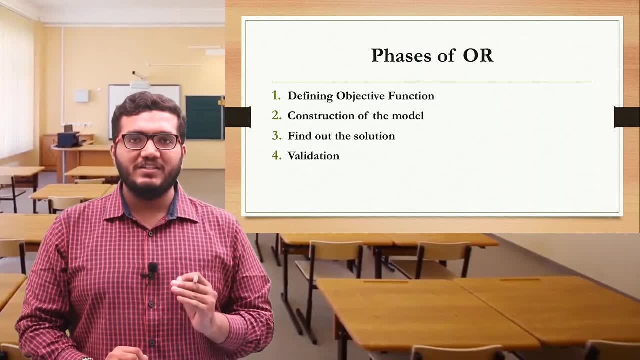 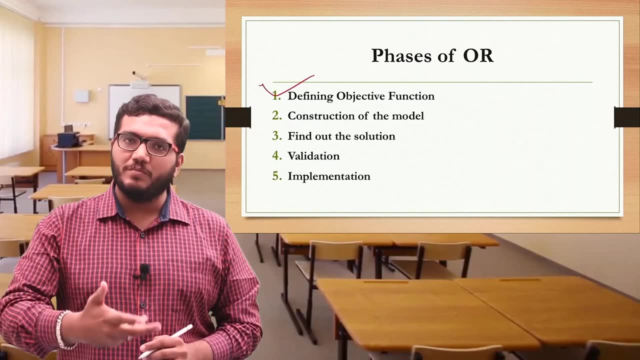 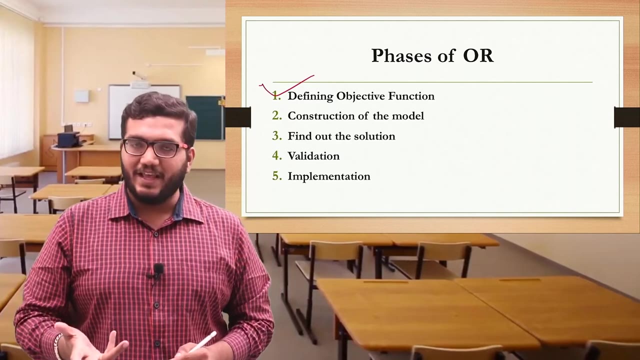 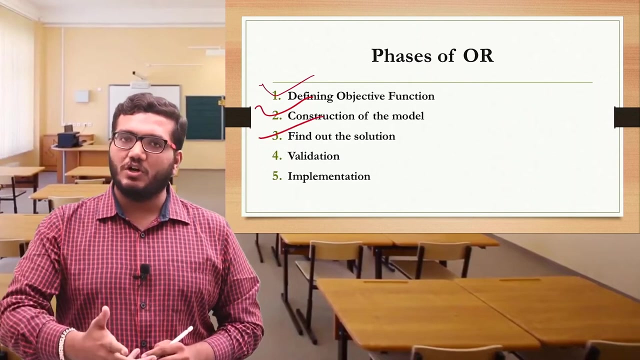 So these are the different five operation research phases. Again, I am repeating: The first step is defining the objective function. It can be maximization type, minimization type or the within the certain range. Second is the construction of the model. After the construction of the model we are going for the: finding out the solution. 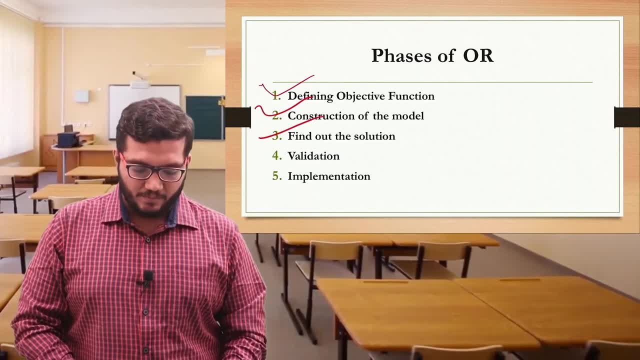 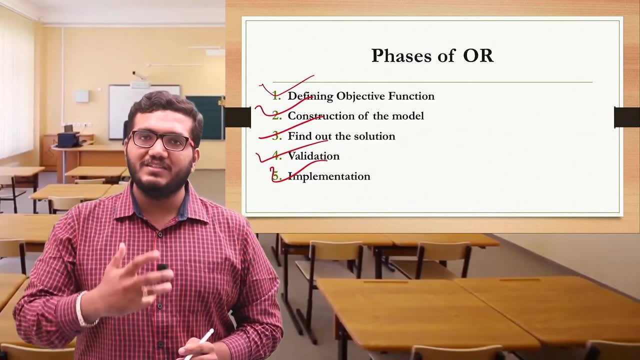 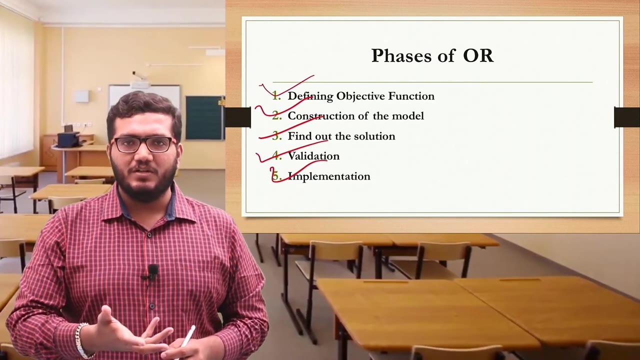 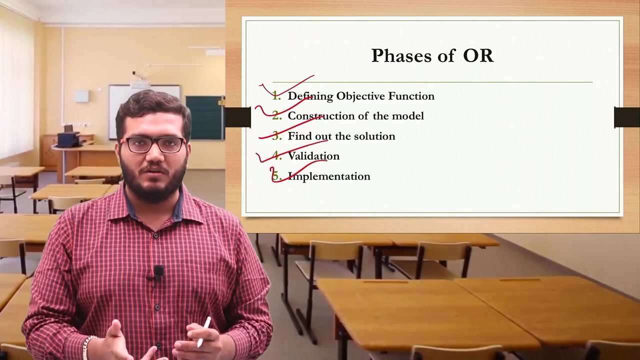 Whatever we have as a solution, that must be valid And the final stage is implementation of it in the real world. So these are the five different phases of the operation research. Now let's take one example So you can have more idea about what operation research and which kind of problem the operation research can solve. 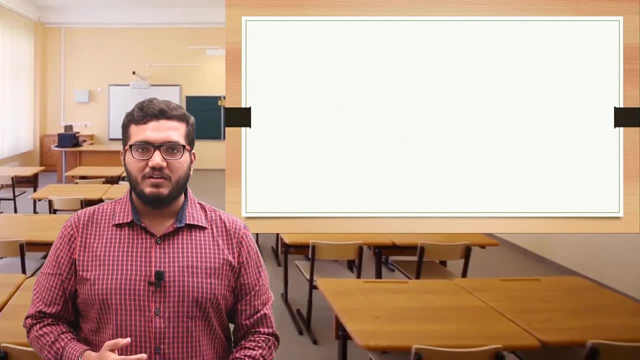 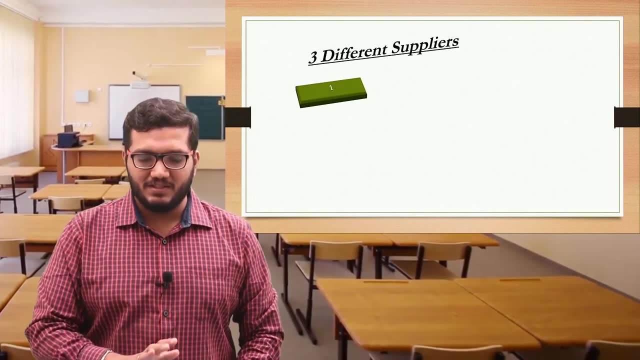 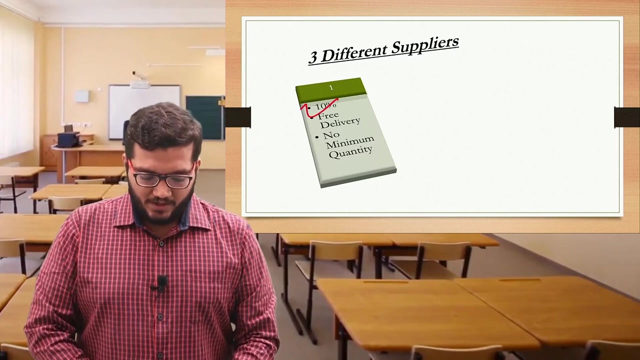 Now we are having three different supplier Supplier one that provides me 10% discount- It doesn't take any delivery charges And the third important thing, That is no minimum order quantity. The next supplier- That is my second supplier, That is- gives me the 20% discount. 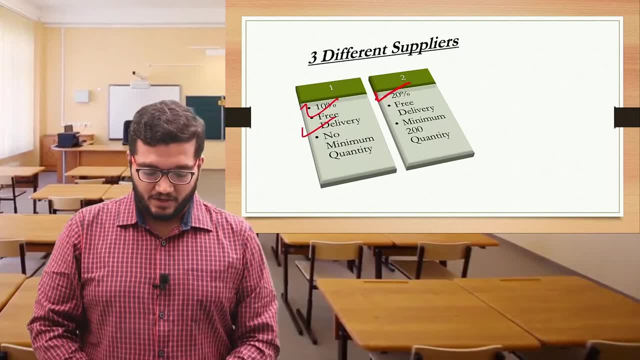 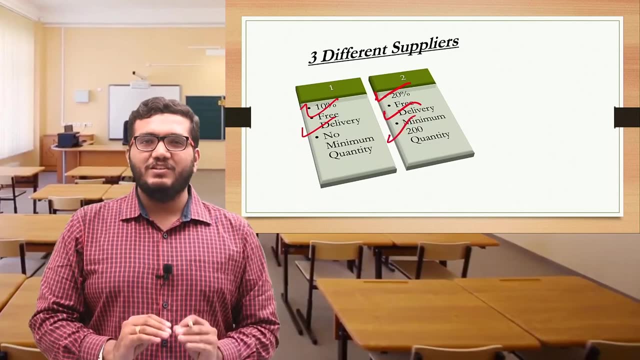 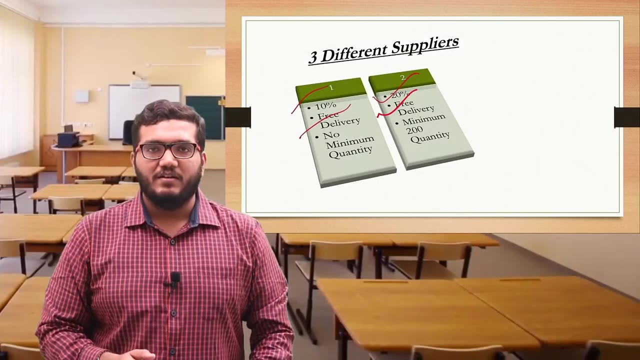 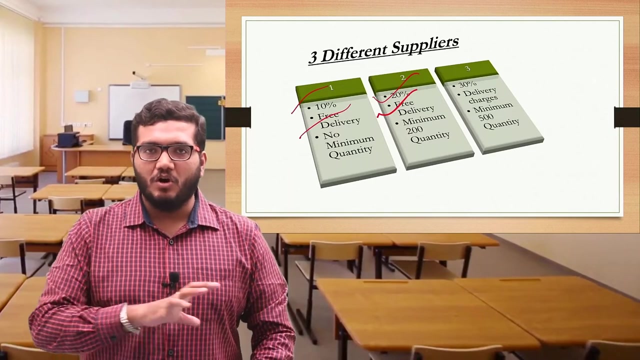 The 10% more discount than my first supplier. Again, it provides me free of cost delivery. And again there is one change. The change is I need to buy minimum 200 quantity from this supplier And my third supplier. That provides me the 30% discount that is maximum among all these three.